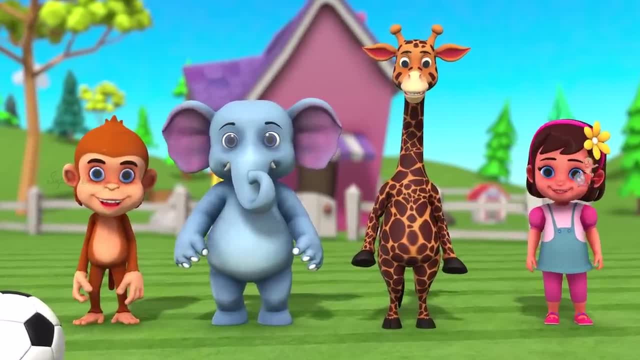 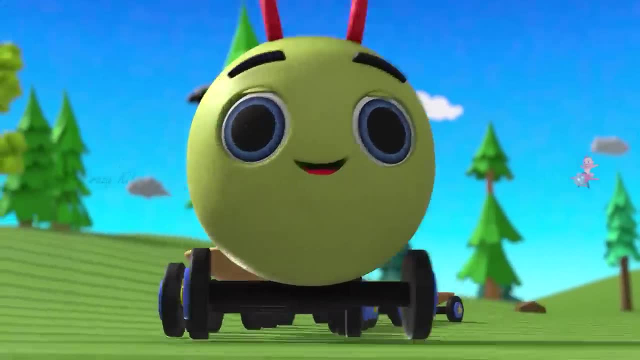 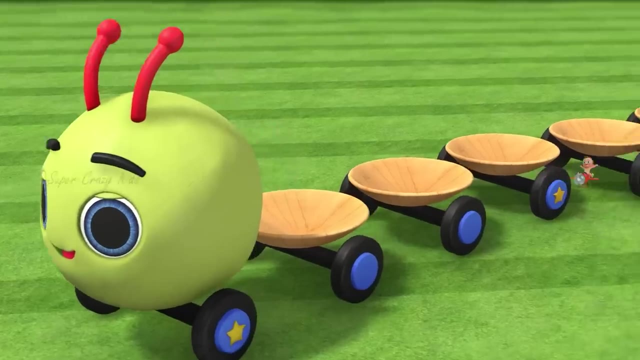 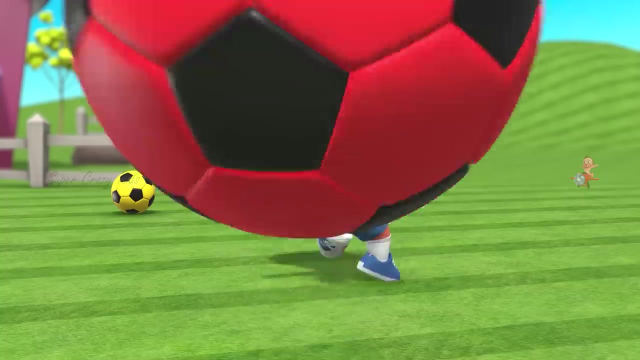 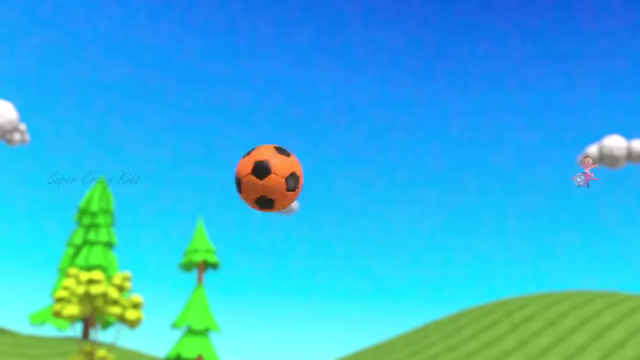 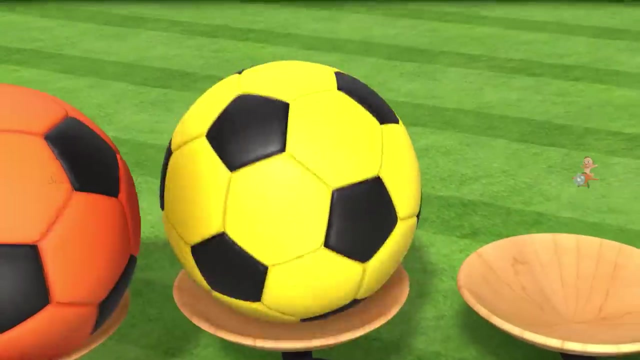 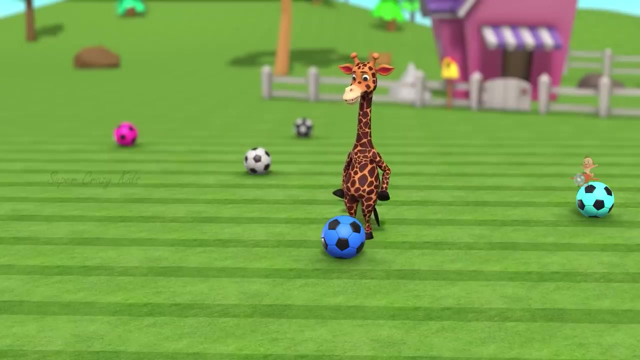 That sounds good to me. Let's play. Wow, I love it. Amazing, Looks, interesting. Here we go. Yahoo, Red color, Look here. Orange color, Hey Bananas, Come on. Yellow color, Green color, Hmm, This is funny. 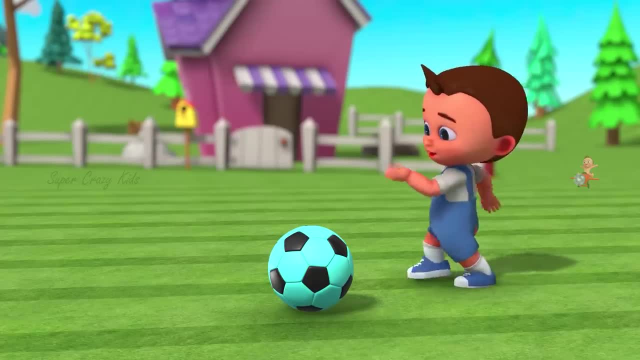 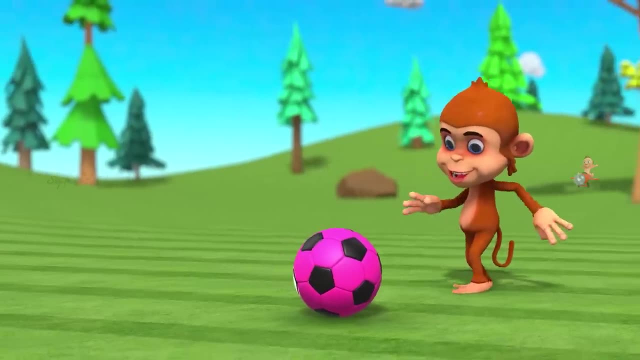 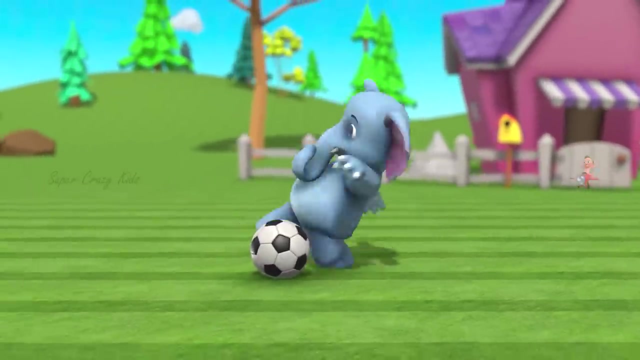 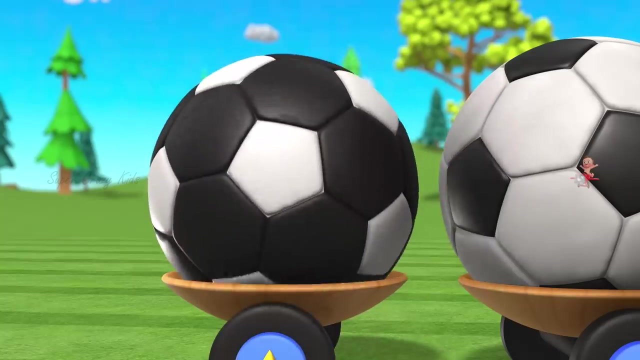 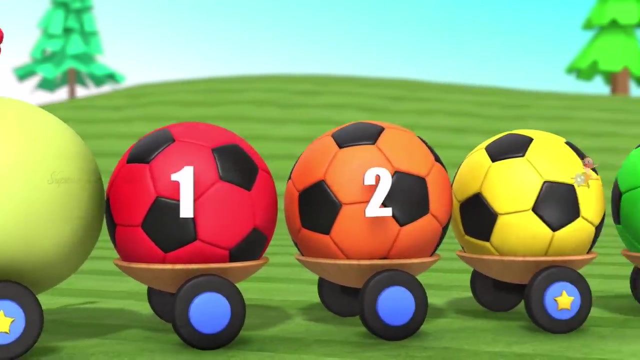 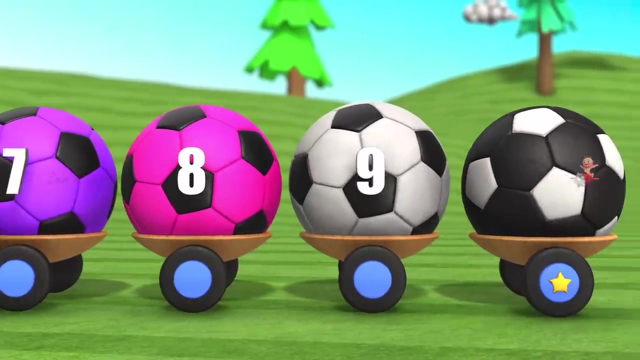 Blue color, Yahoo, Cyan color. Purple color, Pink color, Woo-hoo Woo-hoo. White color, Black color- That is awesome. One, two, three, four, five, six, seven, eight, nine, ten. 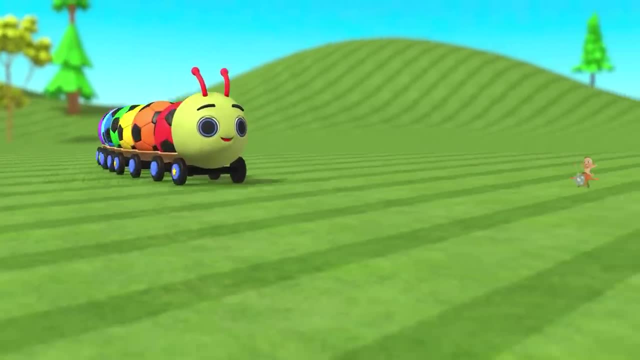 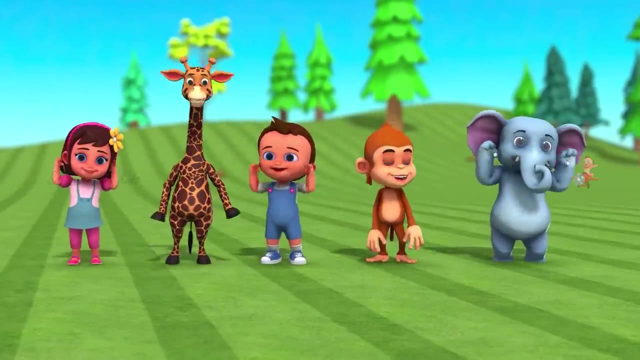 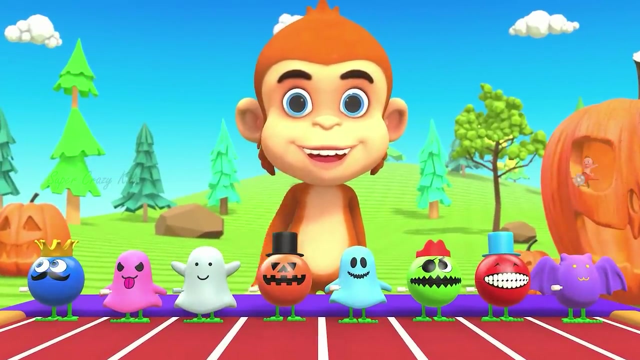 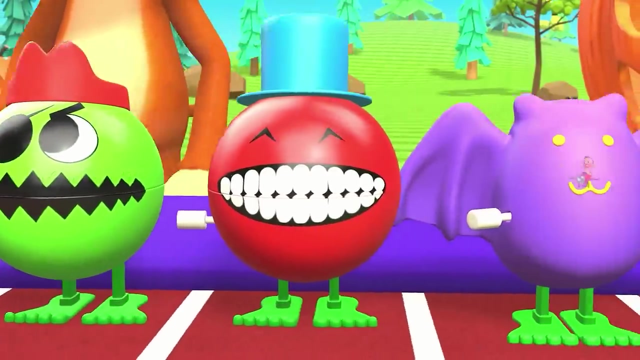 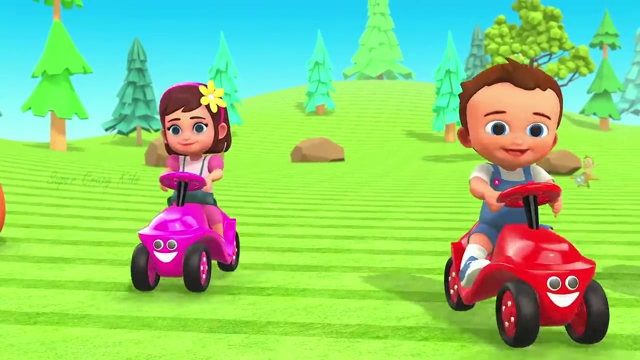 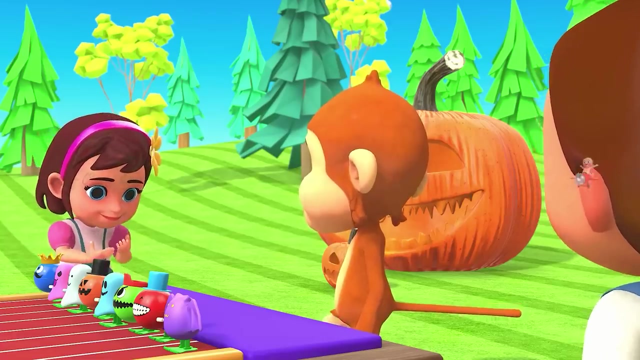 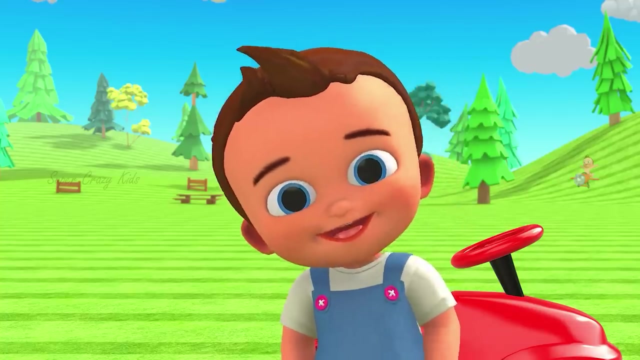 Wow, Wow, That was wonderful. Bye, Hello friends. Look over here. Oh, wow, Amazing, Looks interesting. Hey, Hey, Look at this place. Hey, What's going on? Did you see that? Okay, Let's do this. 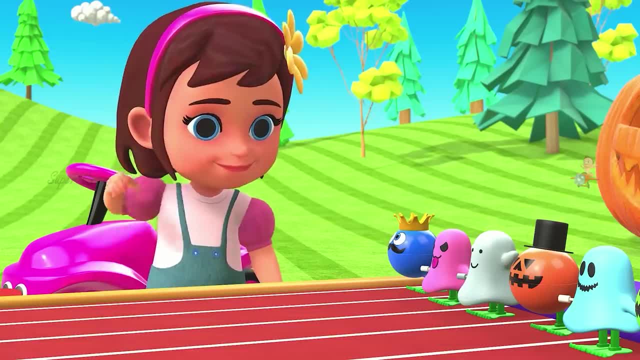 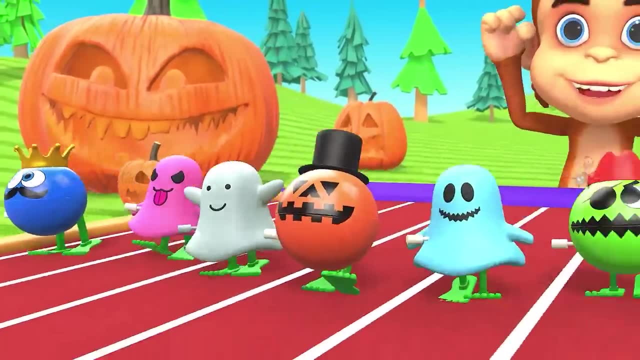 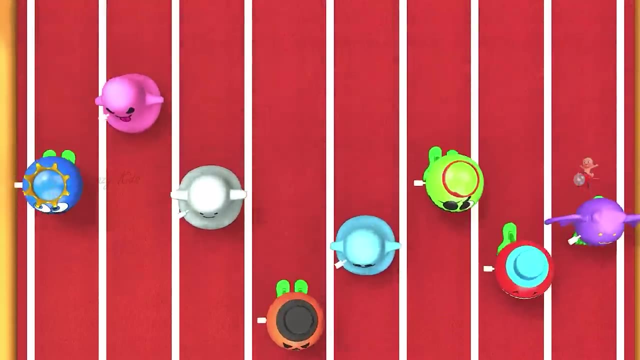 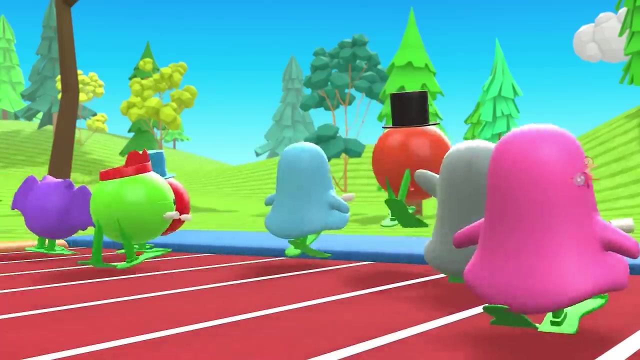 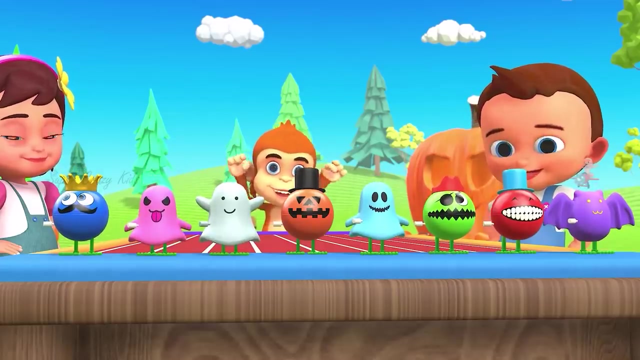 Hey, Watch out Yahoo. Hey, Come on, That is awesome. Yahoo, There's another one. If you want to see it, you have to watch it. This is great, Here you go. Alright, You have it Perfect. 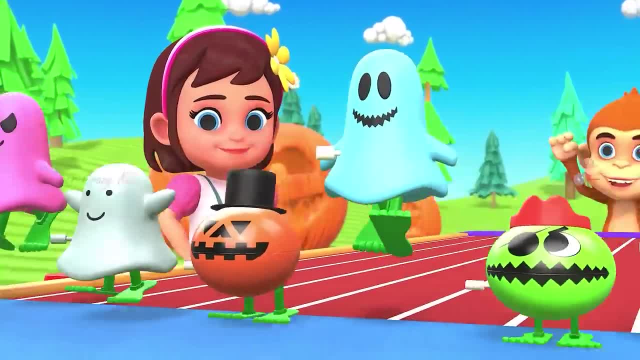 This is awesome, Absolutely awesome. So I have a big idea. Let's see what's here. Okay, Take a look. It's like you know space. I can write down everything. It's like I can put a link to it. 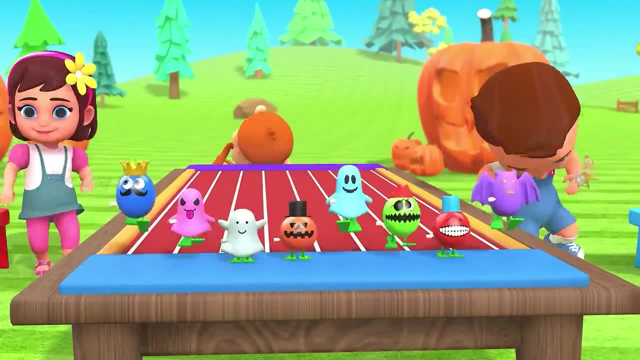 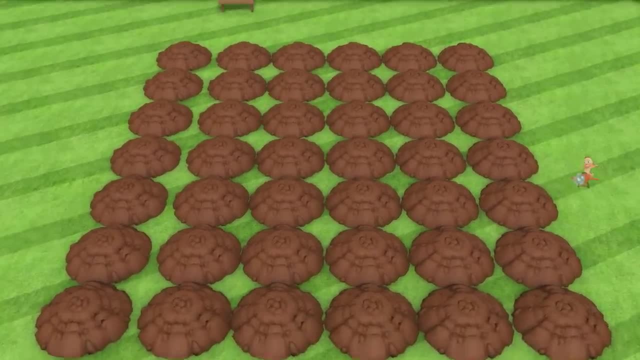 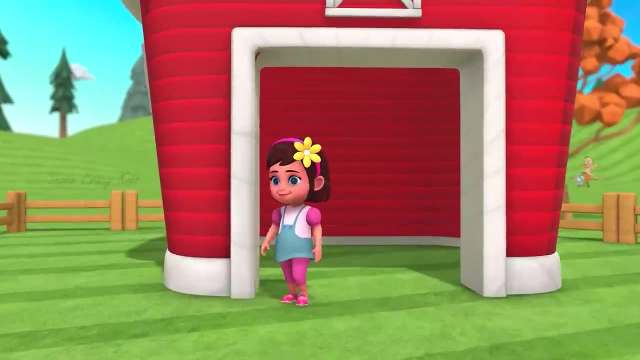 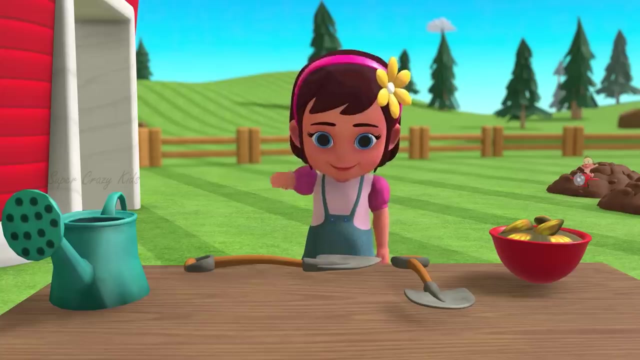 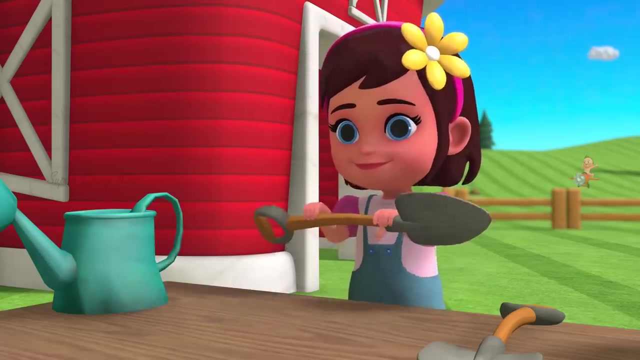 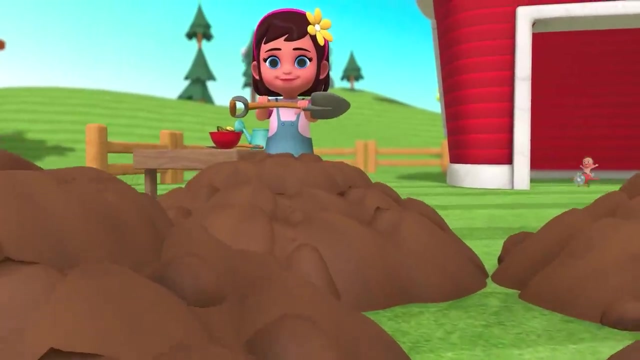 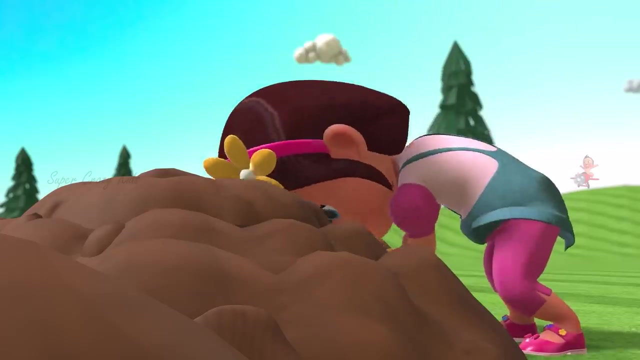 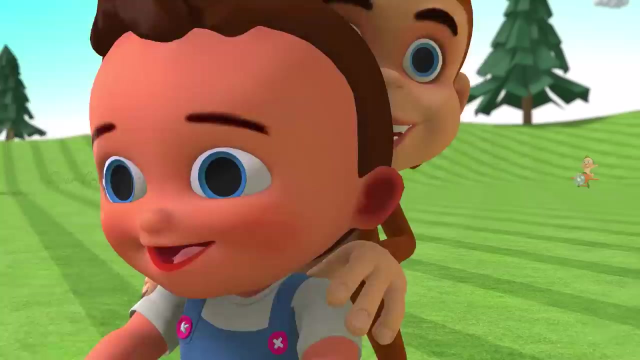 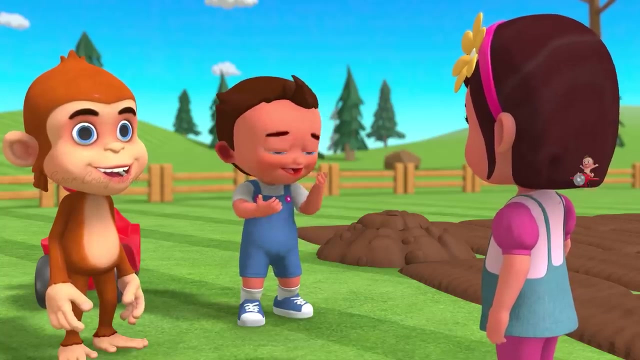 I can put it. I can put it: See Who is that? Look over here, Hello friends, Let's go over there. Oh, wow, Okay, let's do this Ouch. Hello friends, What's happening here? Well, Hello, Hello friends. 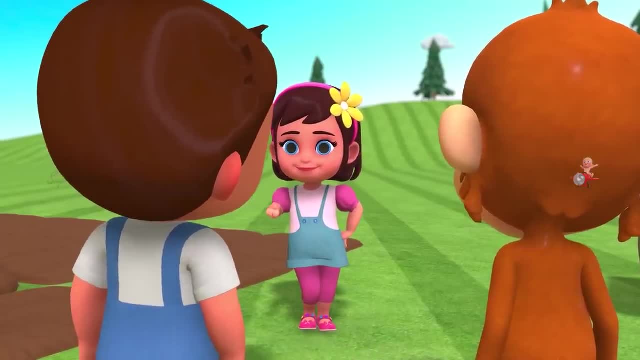 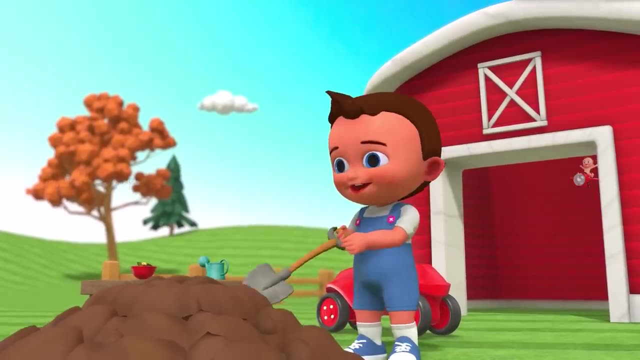 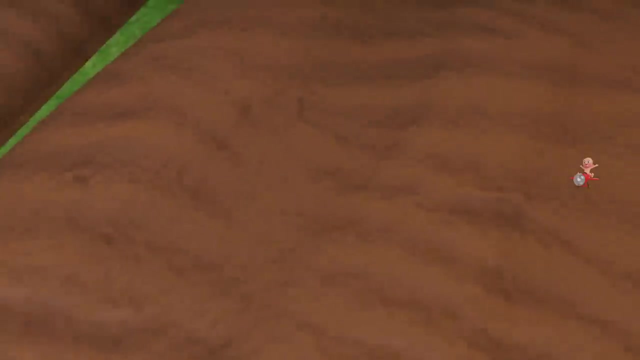 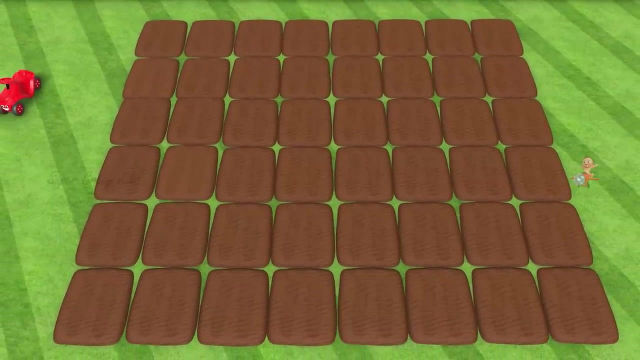 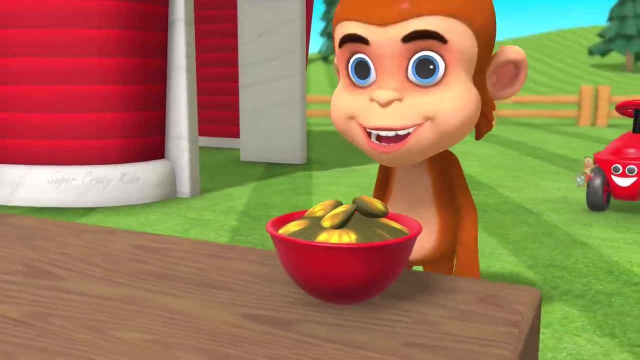 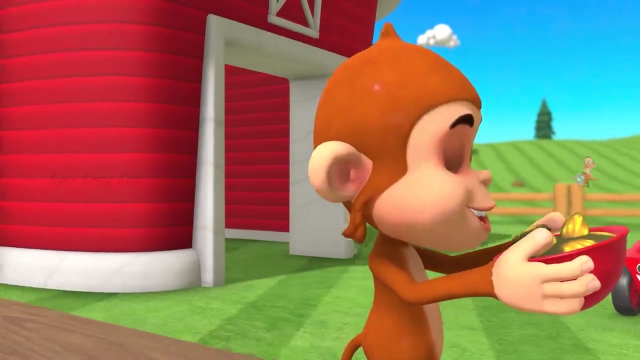 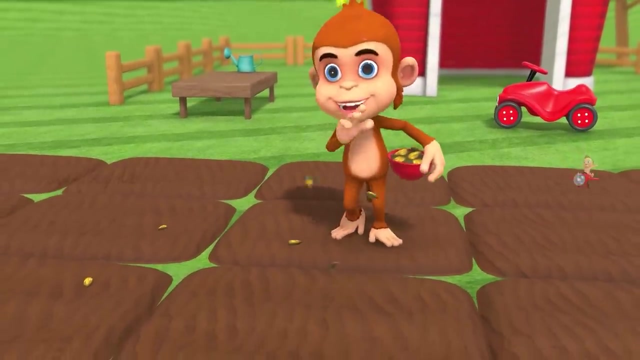 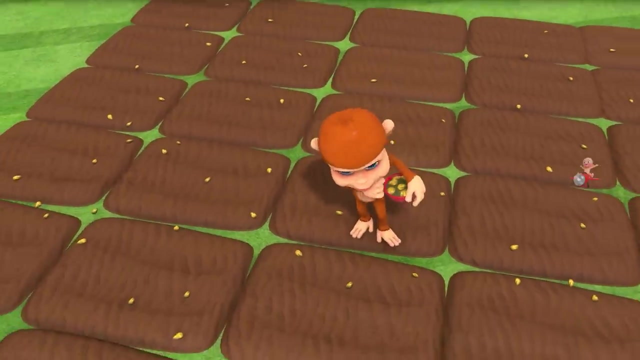 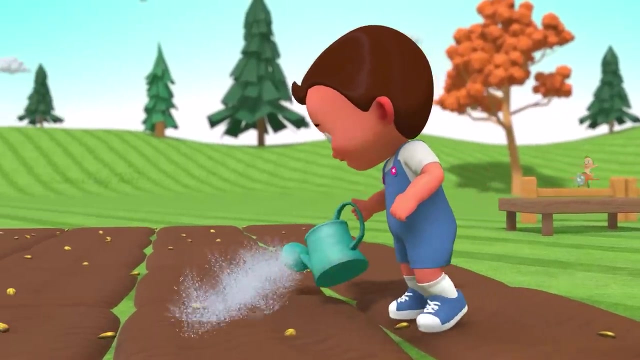 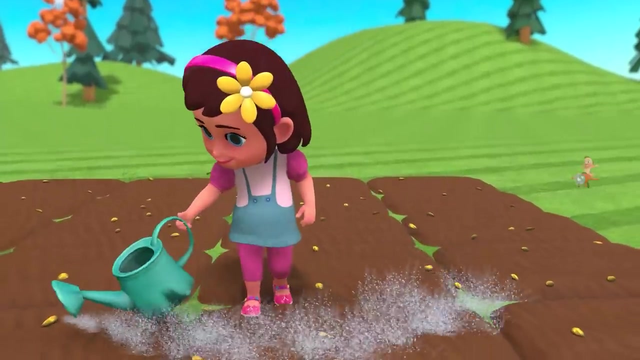 That has a plan for today. I will show you how Let's go. Yeah, let's go. Oh, wow, Amazing, looks interesting. Now it's your time. Hey, bananas, Let's go over there. This is funny. Let's go over there. Let's go over there. 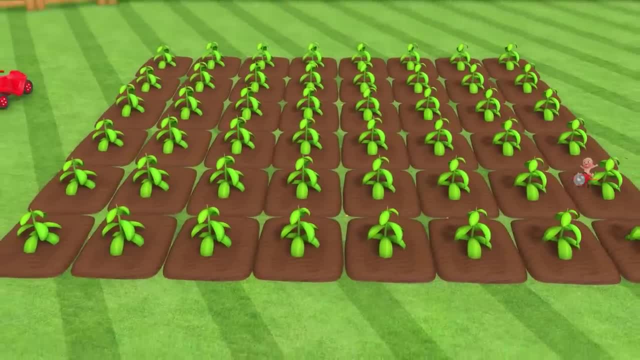 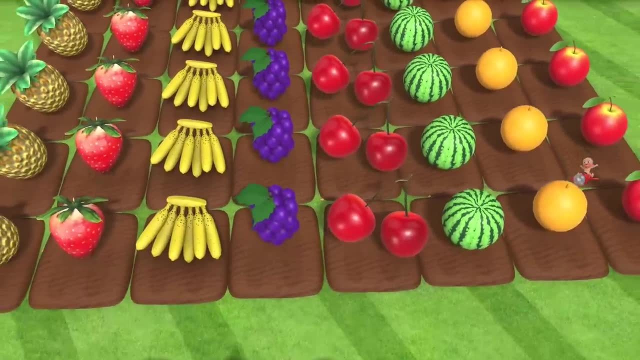 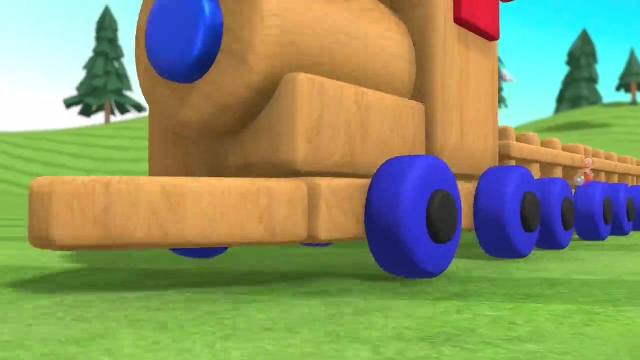 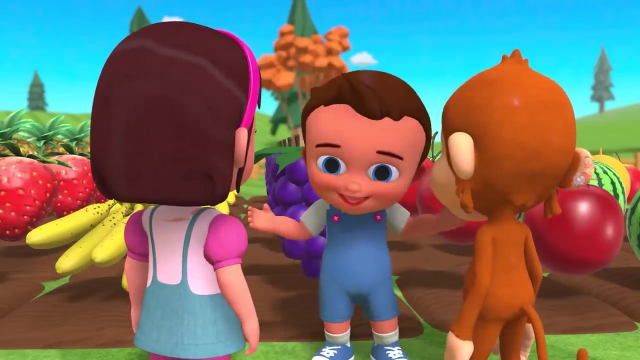 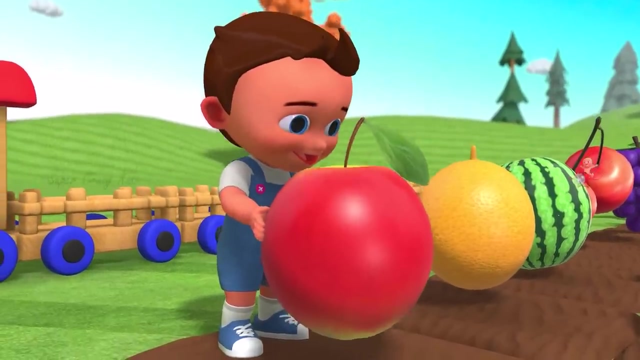 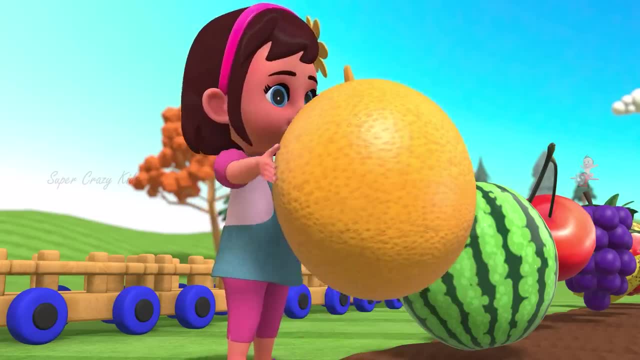 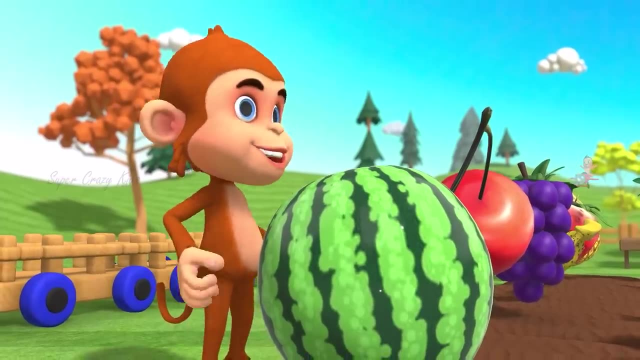 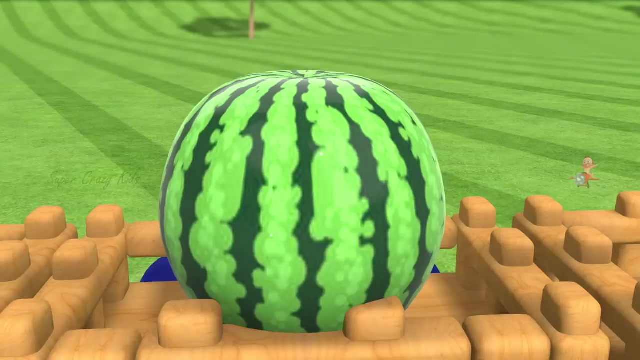 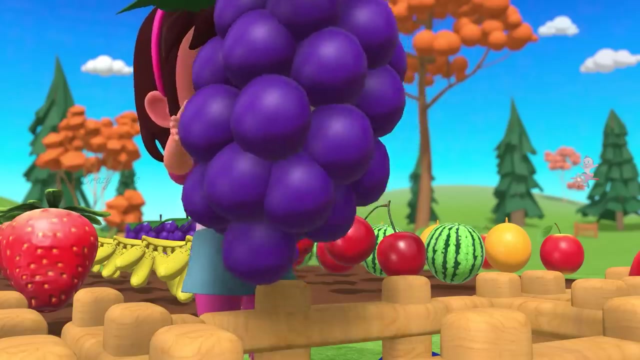 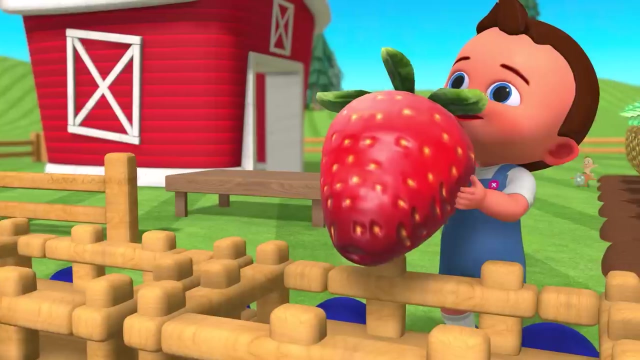 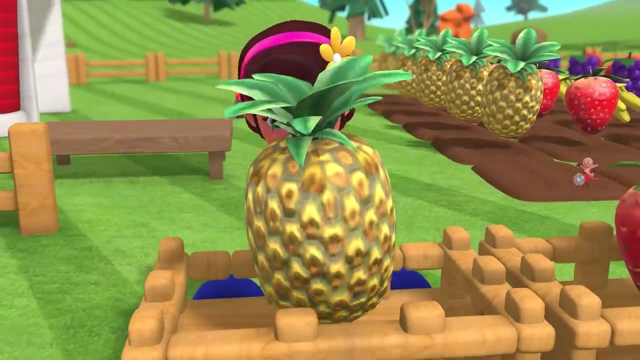 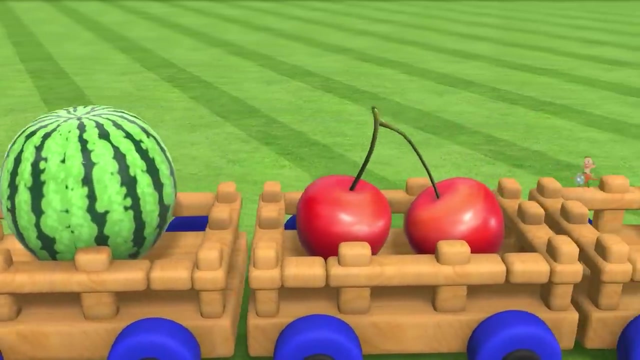 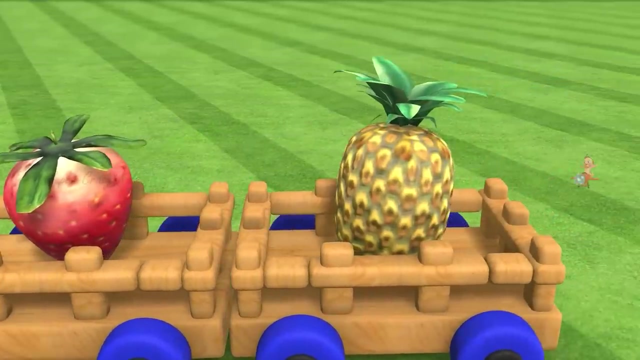 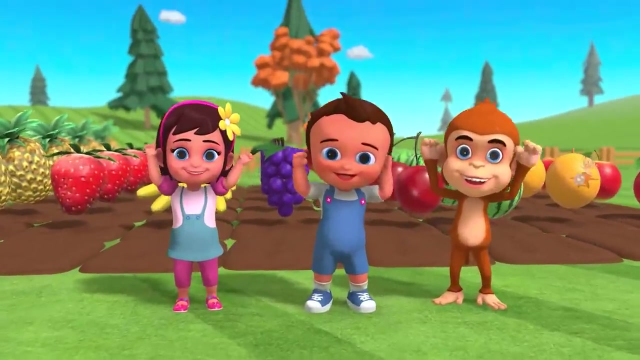 Apple, here we go. Do you know what fruit? this is An orange, Watermelon, Cherry, Grape, Banana, Strawberry, Pineapple. That looks fantastic. I love it. I love it. That was wonderful. See you guys. 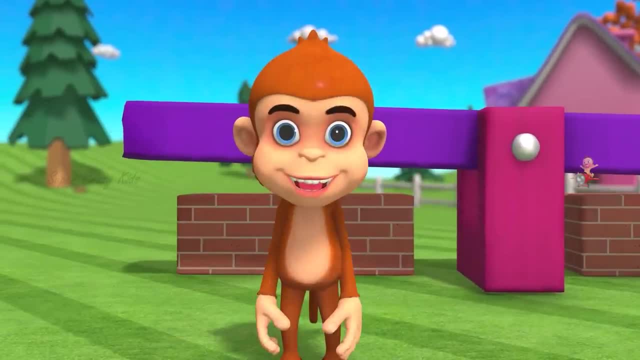 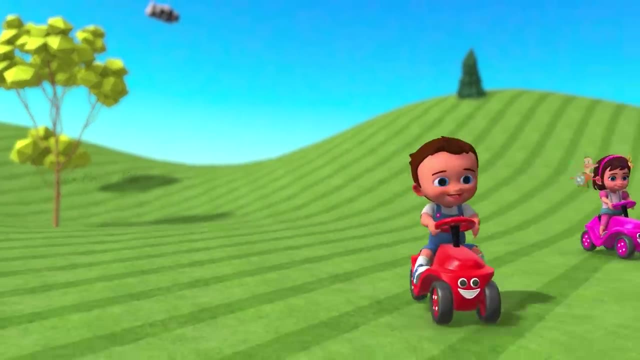 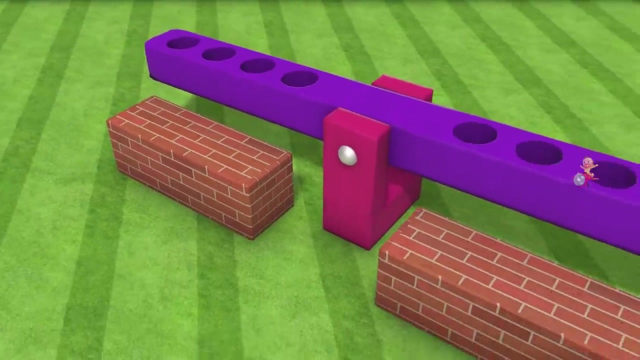 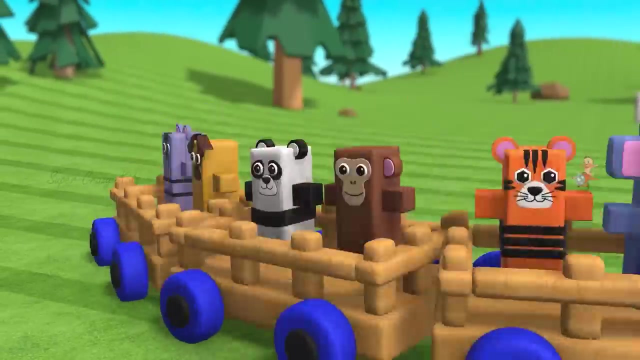 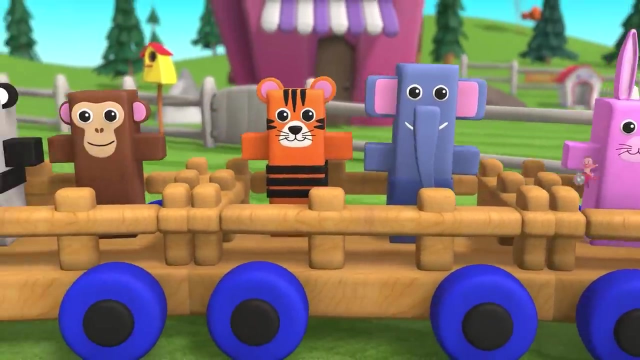 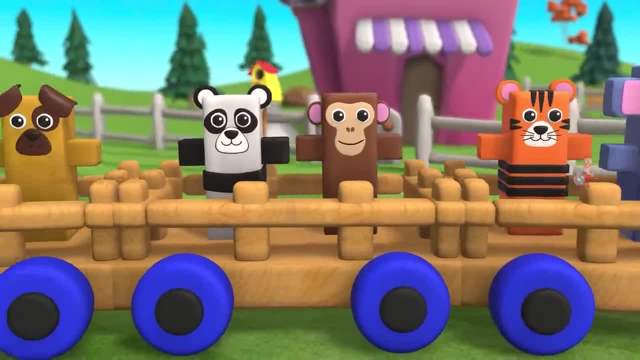 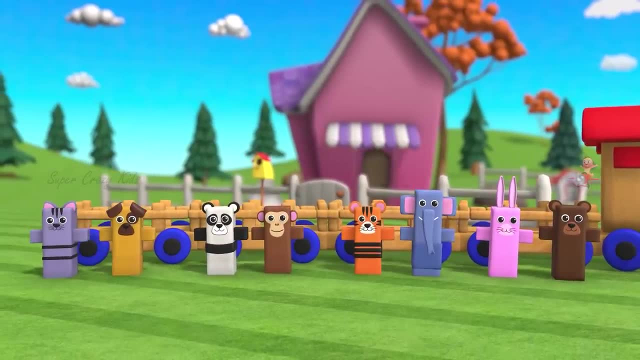 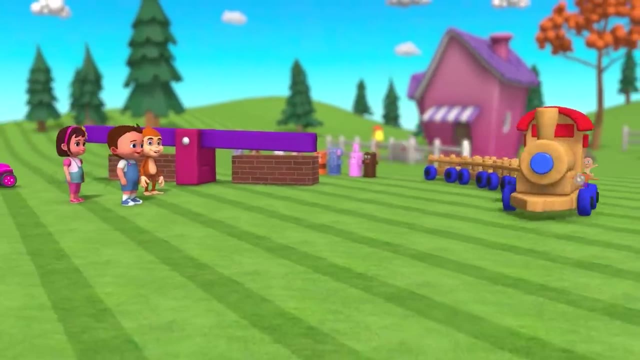 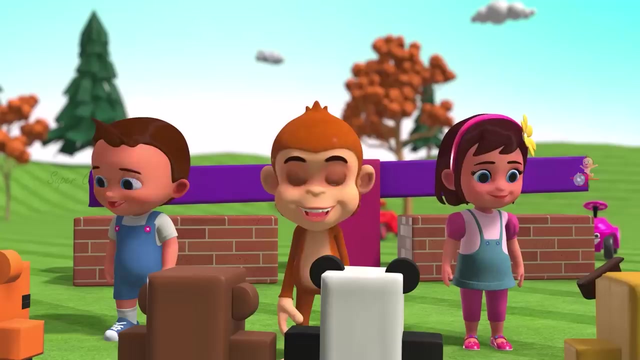 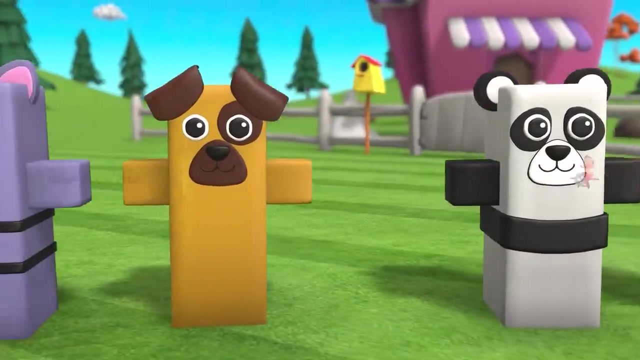 Have a look here. I think this looks so much fun. What's going on? Do you know what symbol this is? This is Train. Hey Bananas, These animals look interesting. What shall we do next? I will show you how to play. Let's go. 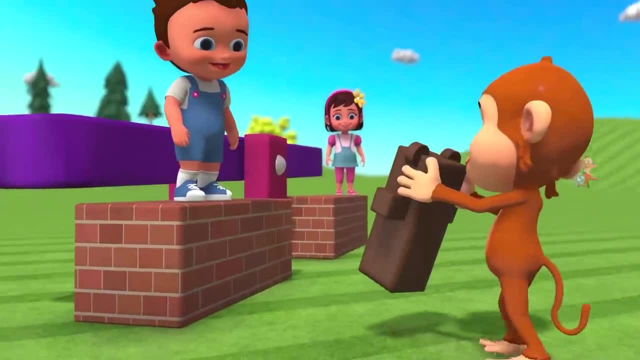 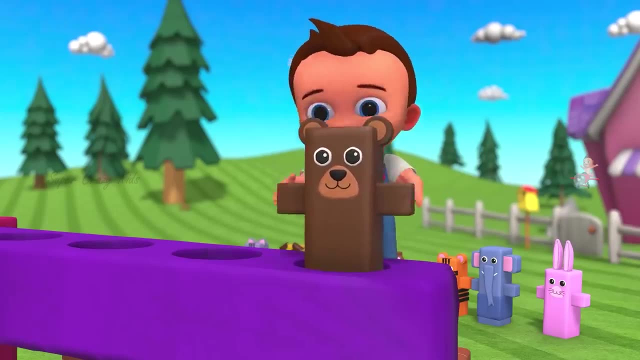 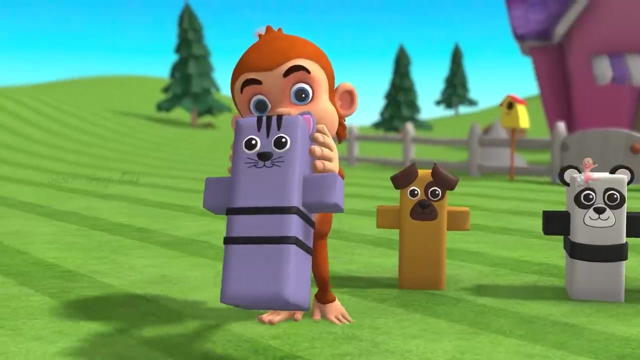 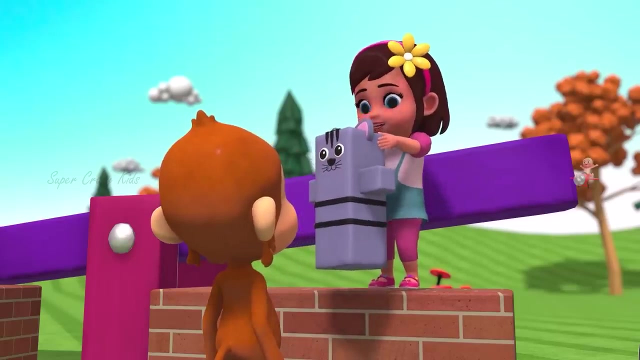 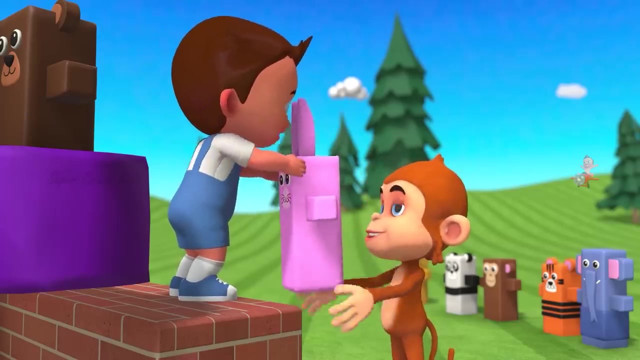 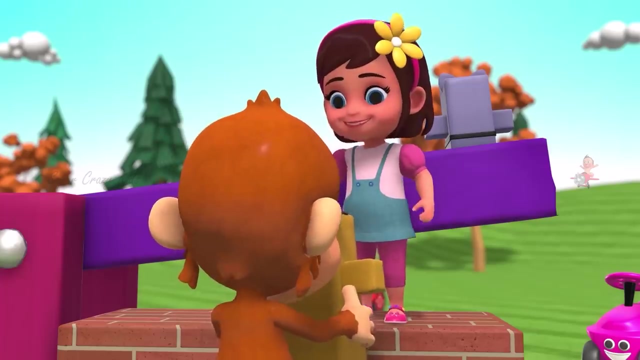 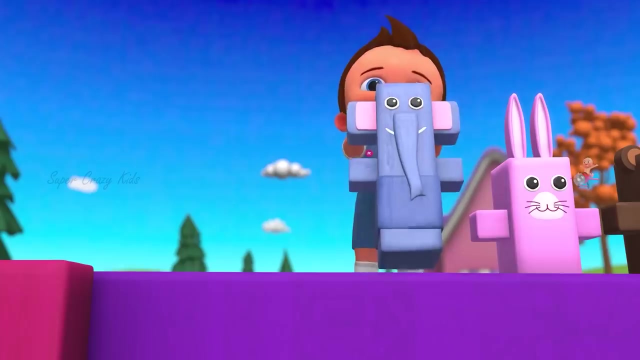 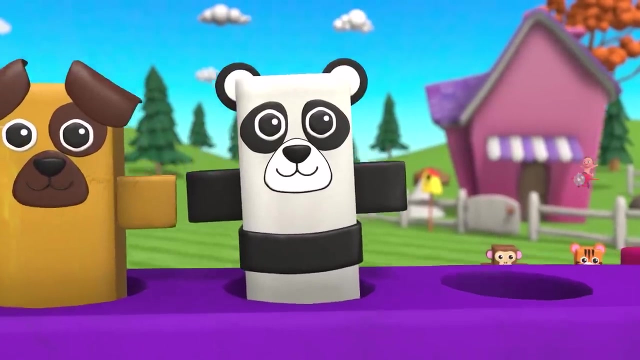 Woohoo, Yeah, Over here. This is fair, You are genius, Good one. This is cat. Woohoo, This is rabbit. That looks fantastic, Perfect. This is dog. This is an elephant. This is panda. 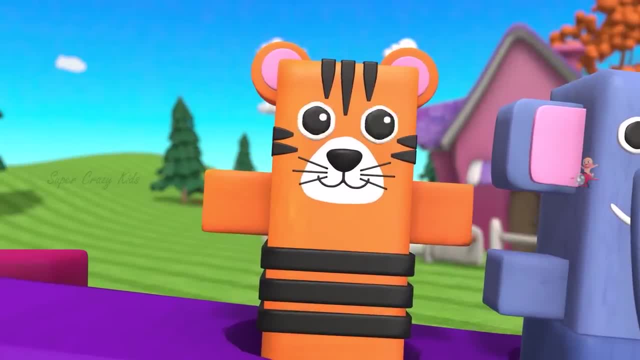 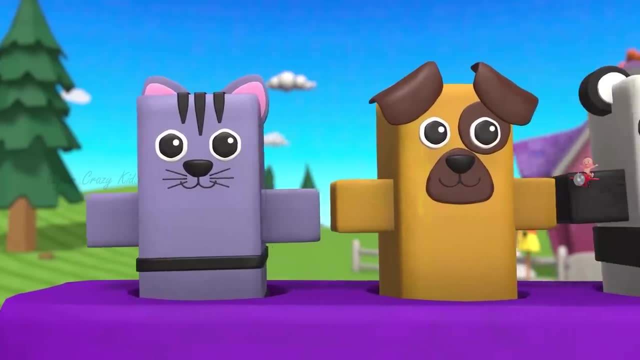 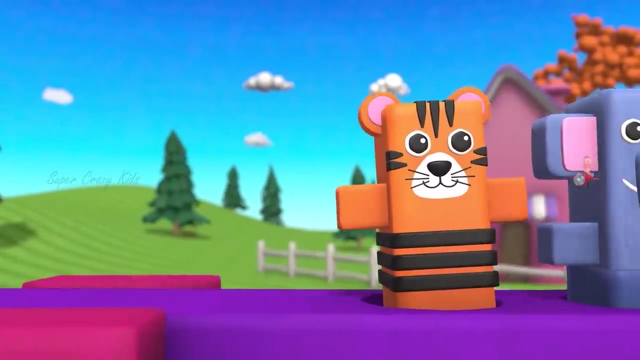 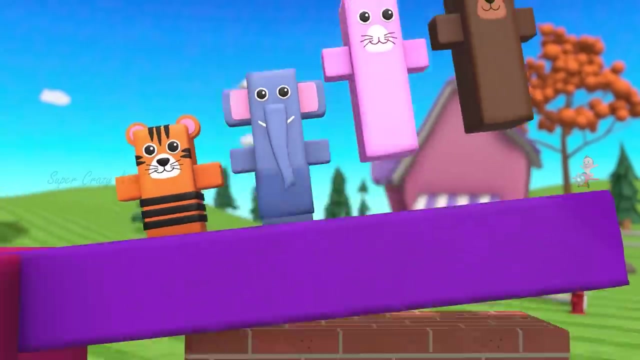 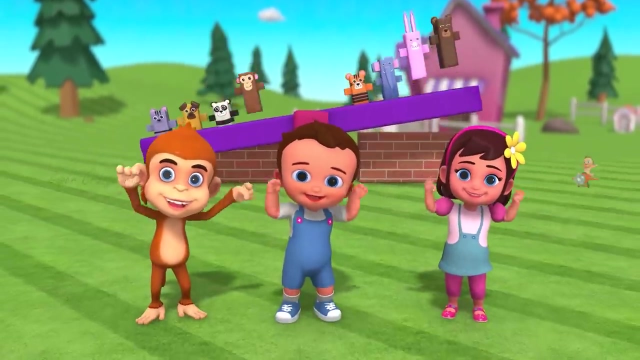 This is tiger. Wow, This is monkey. Here we go. Whoa. Great job, friends. That was fun. That was fun. That was fun. That looks fantastic. I'm so proud of you, So I will see you next time. Bye. 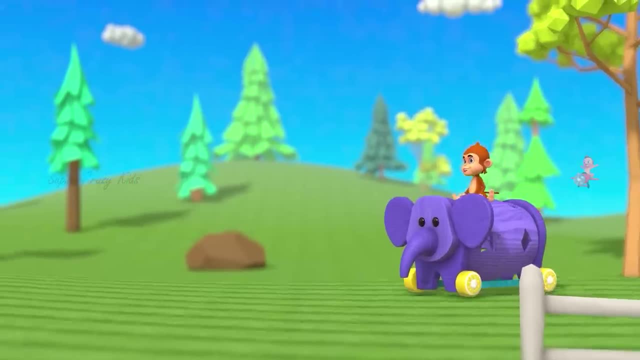 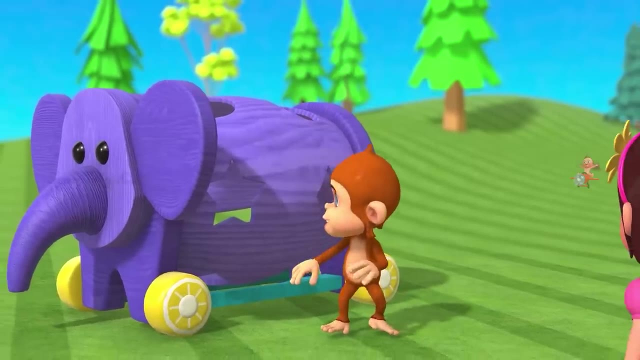 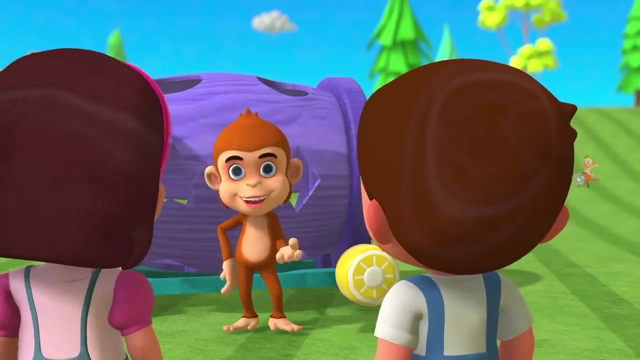 Hello friends. Hey banana, Look Cat's over here. Hey banana, Look Banana, Look Banana. Do you think you could help today? You could? Okay, let's do this, Let's go over there. 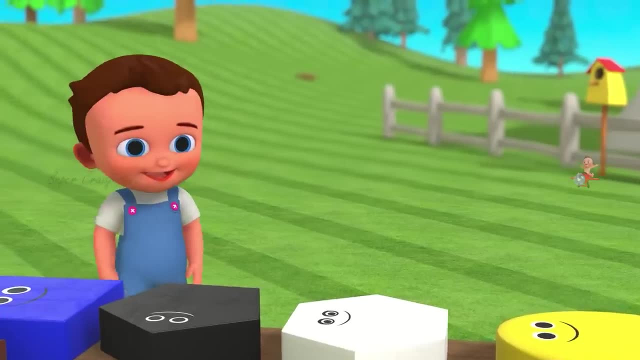 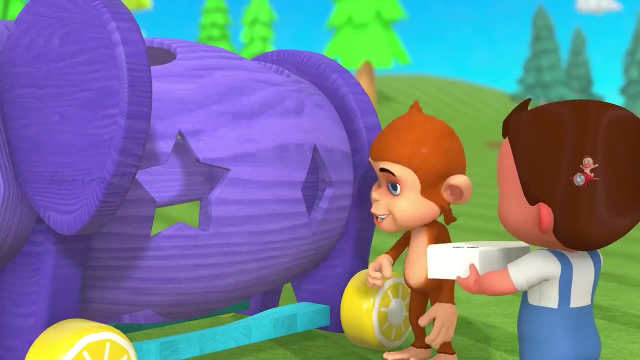 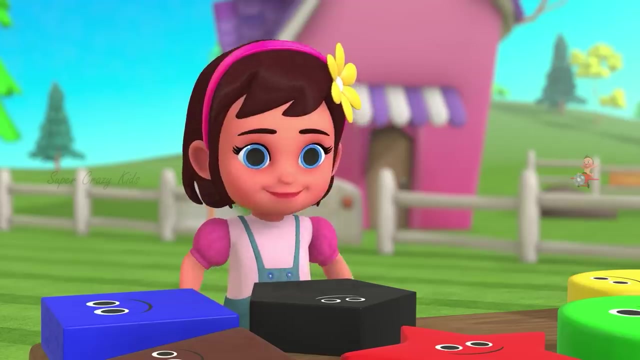 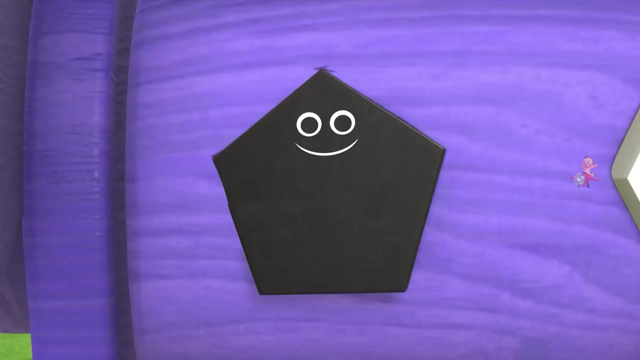 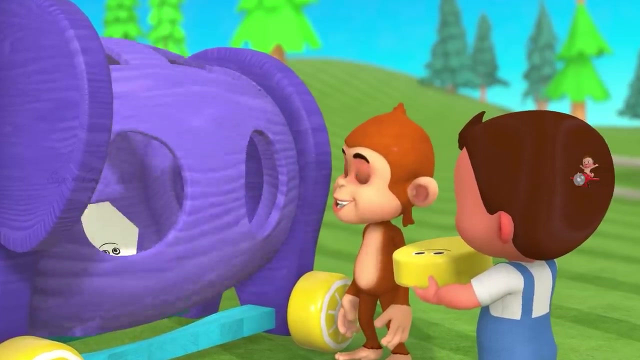 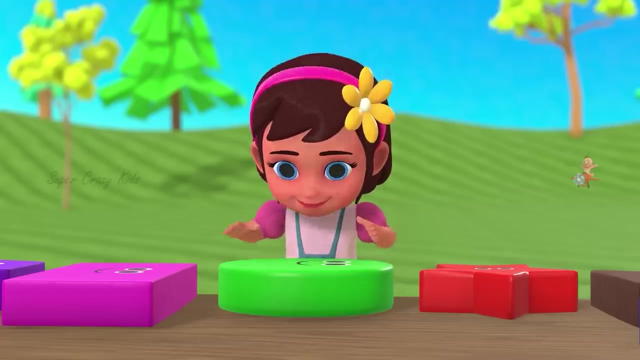 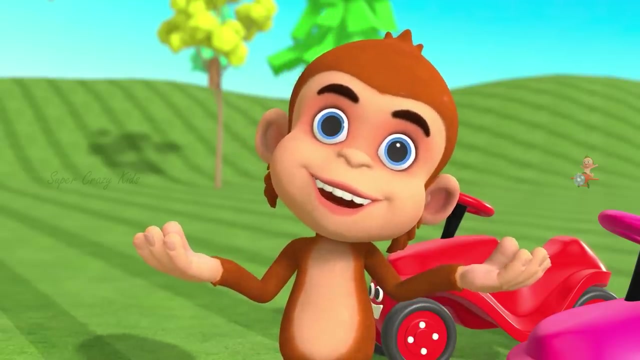 I will show you how. Let's go Watch out. Look over here: Oh wow, Hexagon, Whoa Pentagon, That is awesome. An oval- Oh wow, A circle. That looks fantastic. I'm so proud of you. 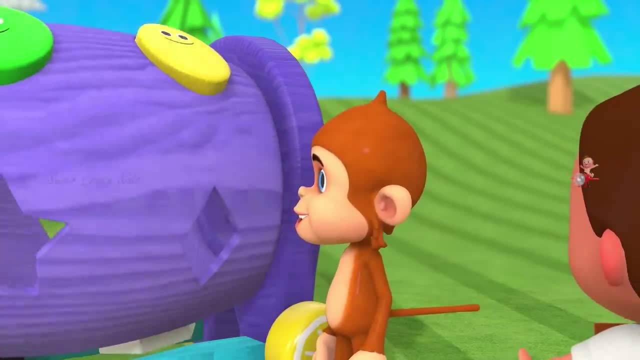 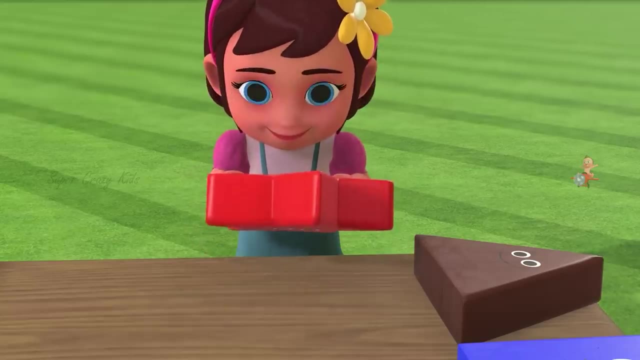 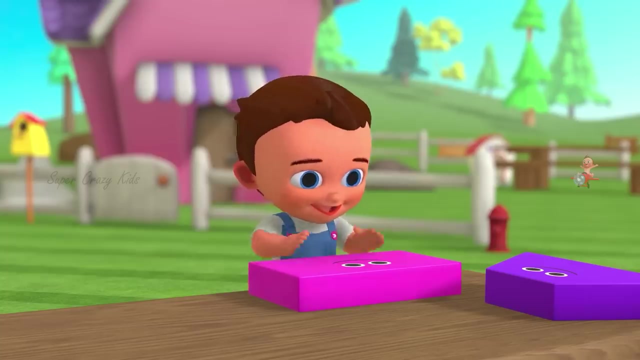 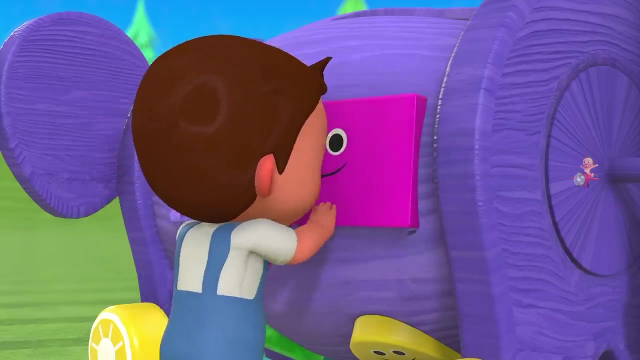 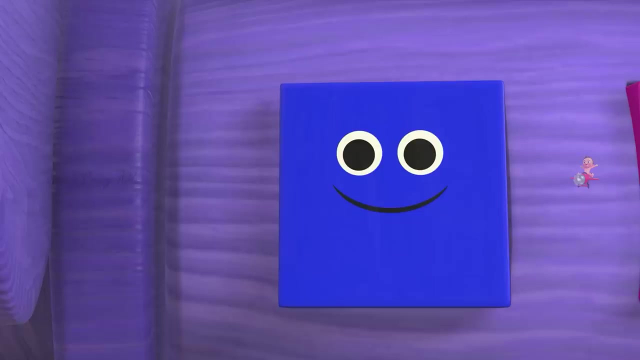 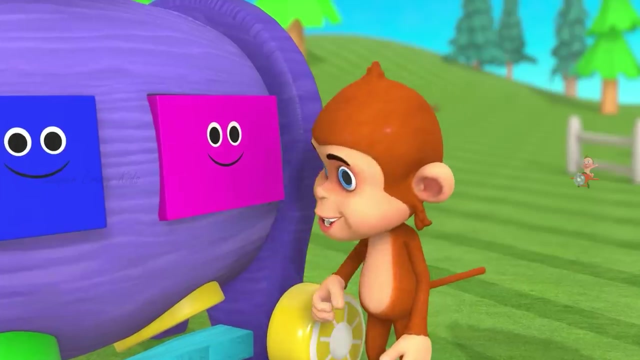 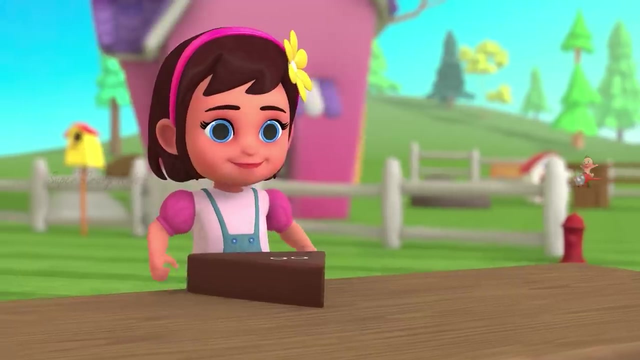 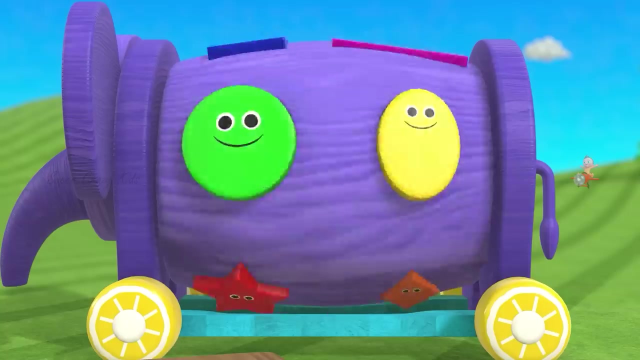 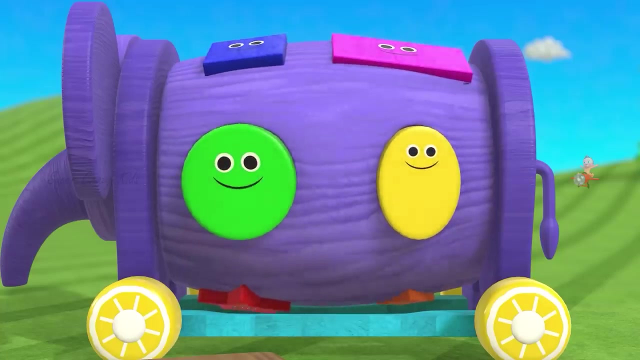 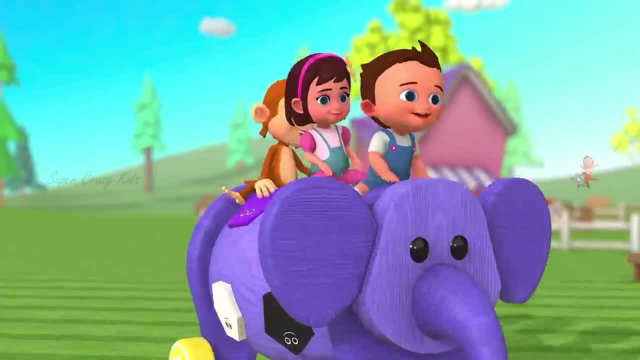 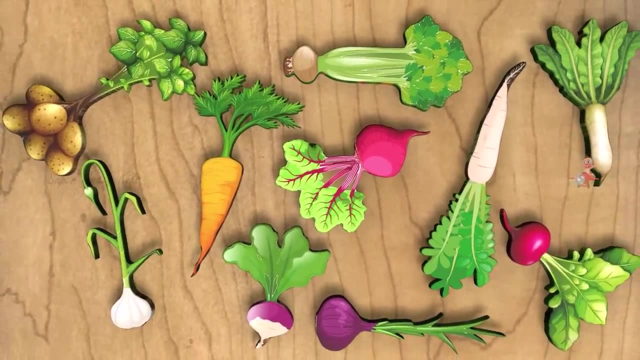 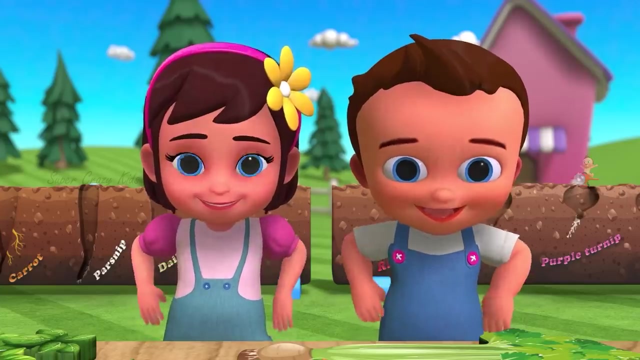 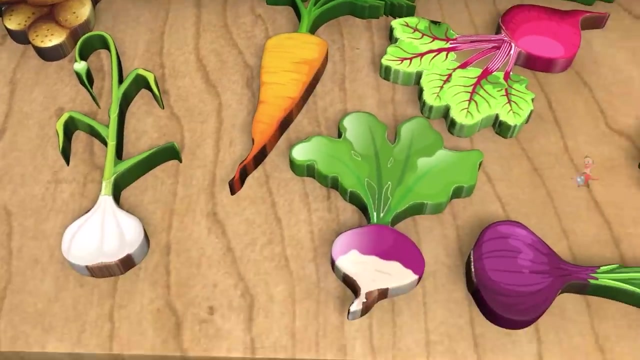 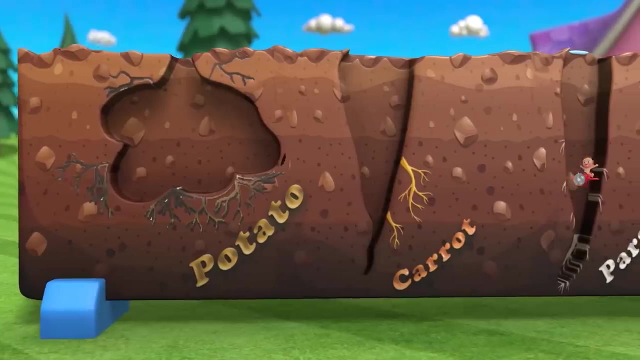 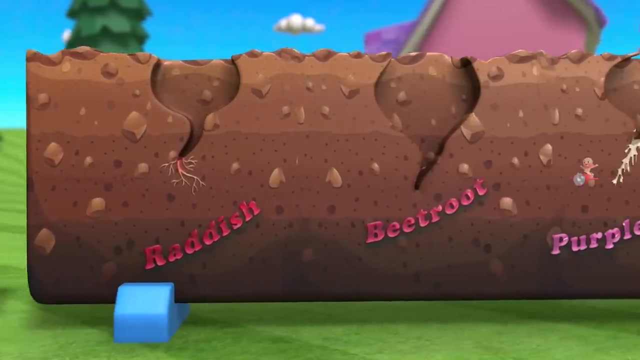 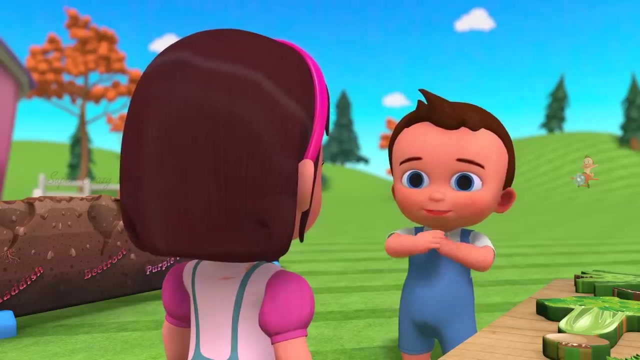 Hello friends, Hello kids. Hmm, what do you think? Yes, we are going to learn vegetables. They look so good. Wow, Look at this place. Awesome, They are going to be so much fun. Today, we are going to be learning about root vegetables. Can anyone tell me what a root vegetable is? Yeah, What are root vegetables? Root vegetables are vegetables that are grown in a garden. Root vegetables are vegetables that are grown underground, like potatoes and carrots. Wow, That's really cool. That's right. 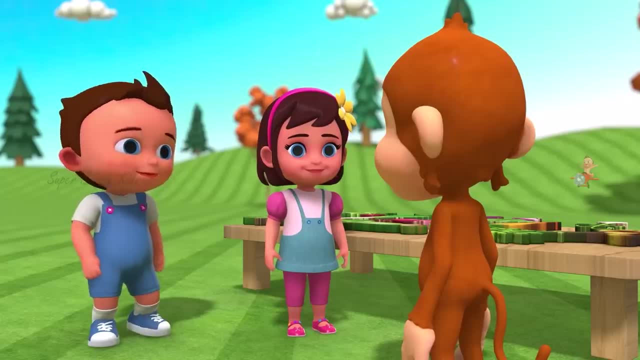 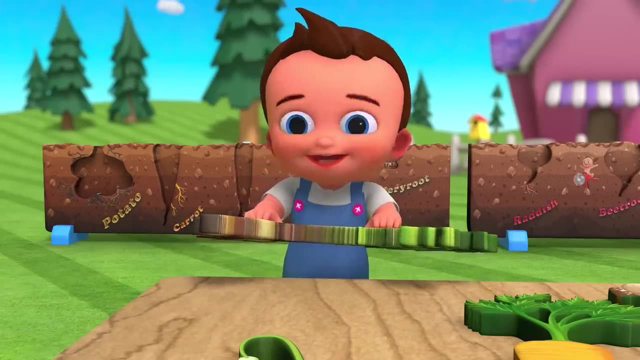 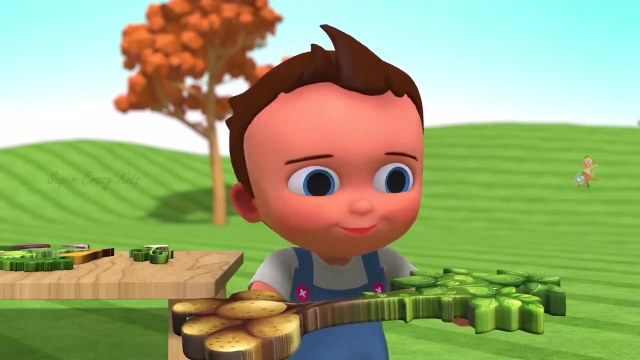 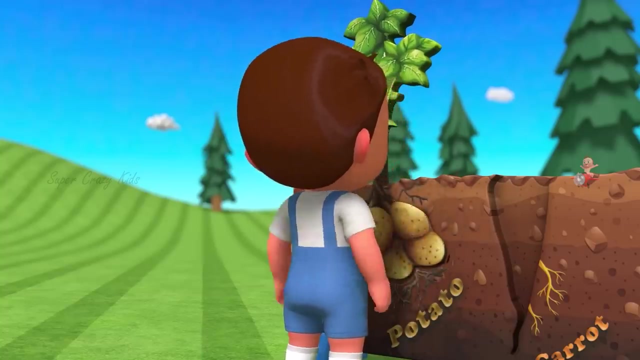 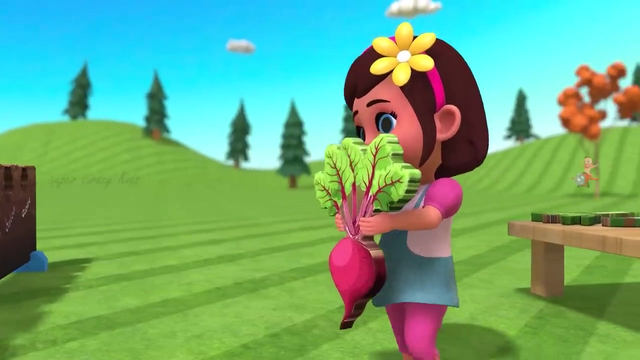 Can anyone name any other root vegetables? Parsnips, turnips and sweet potatoes are also root vegetables. Did you know that pears have many different shots? These are not pears, but potatoes. These are potatoes. Potatoes are potatoes. 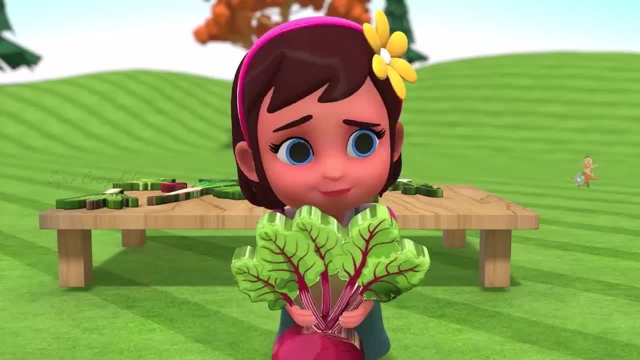 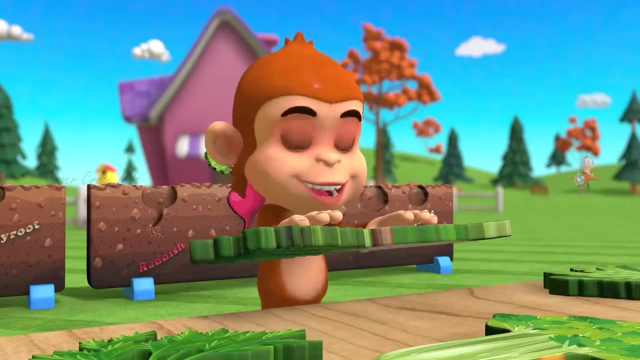 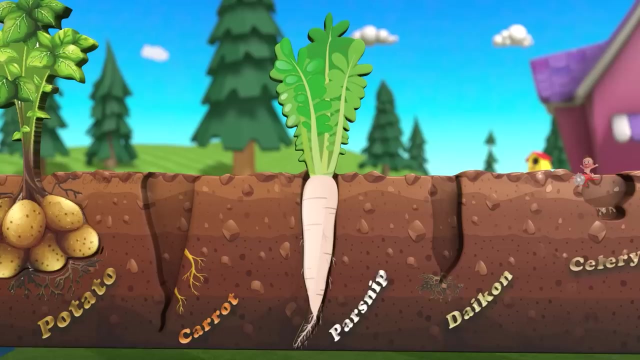 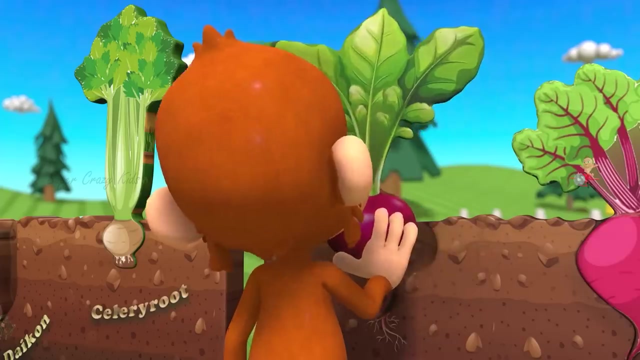 Potatoes always grow bigger if you peel the potatoes or put them into milk. There are many other kinds of soups. Potatoes are goods for your differentiate. This is parsnip, This is carrot, This is celery root, This is radish. 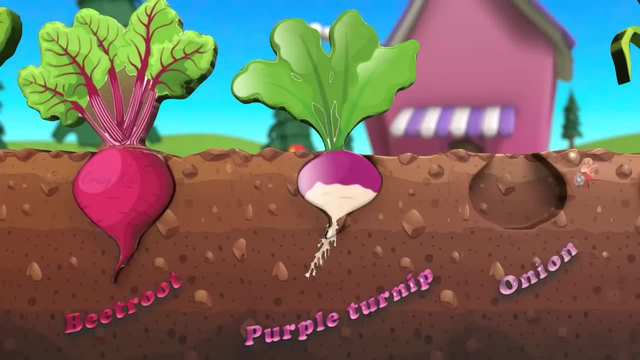 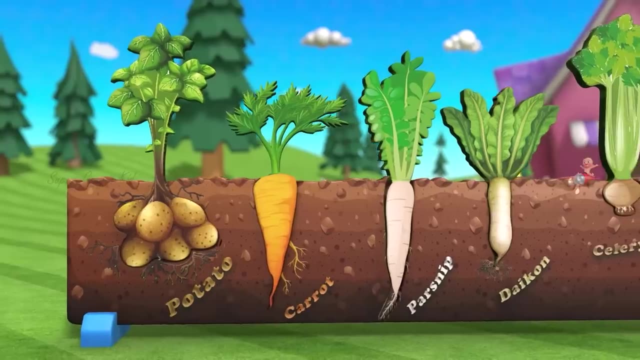 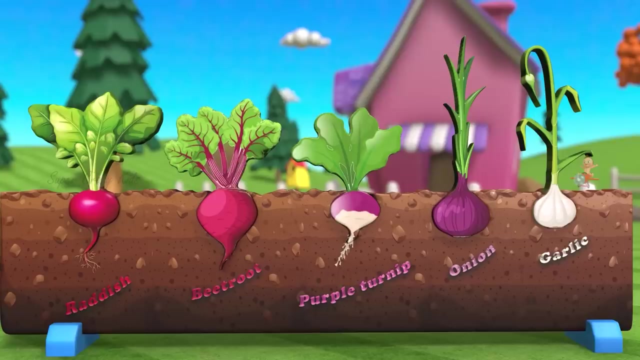 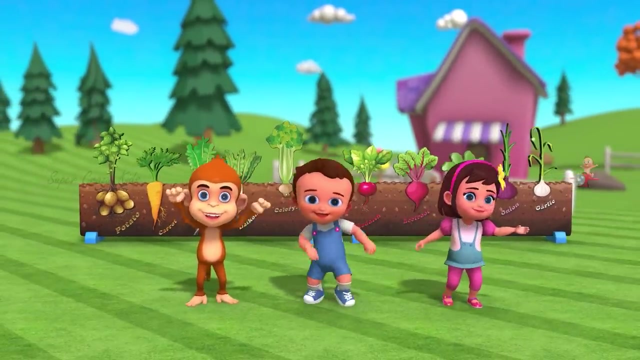 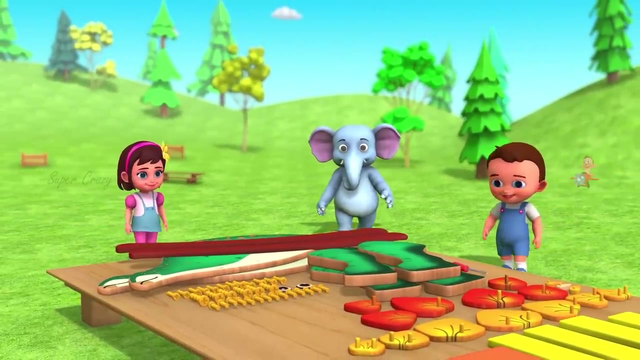 This is garlic, This is turnip, This is daikon, This is onion. Excellent, That's great. Do you have any favorite root vegetables? I love carrots and potatoes, So I will see you next time. Bye, Hello friends. 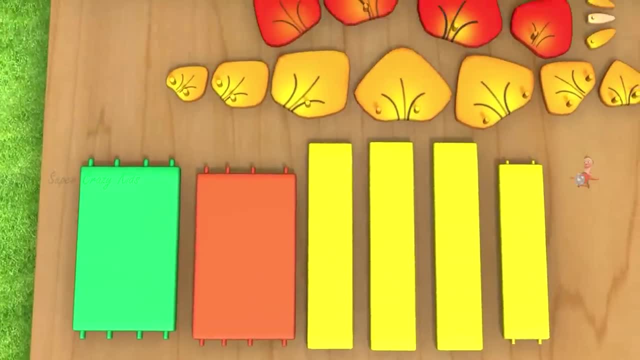 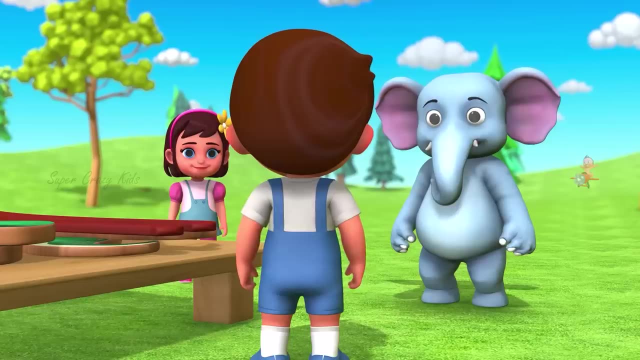 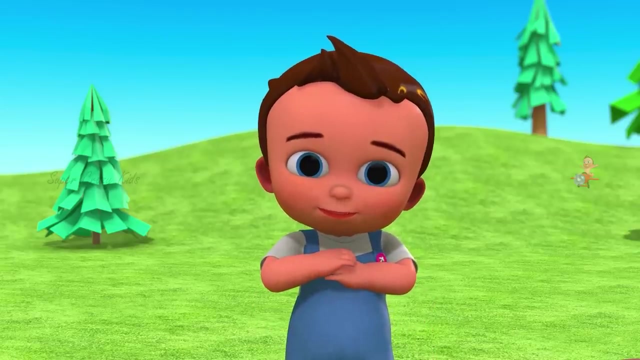 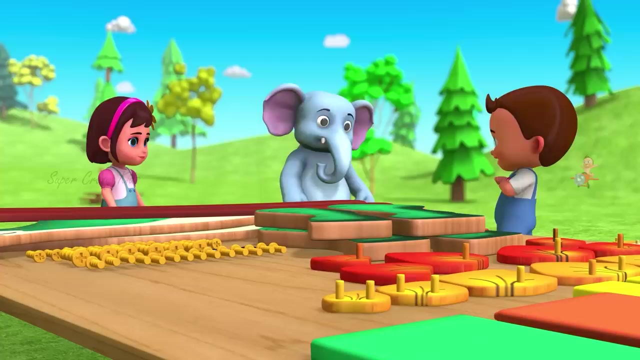 Hmm, What do you think of this video? What do you think Looks interesting? What shall we do next? Yeah, Well, that has a plan for today. Let's look at these first. They look so good. Okay, Let's do this. 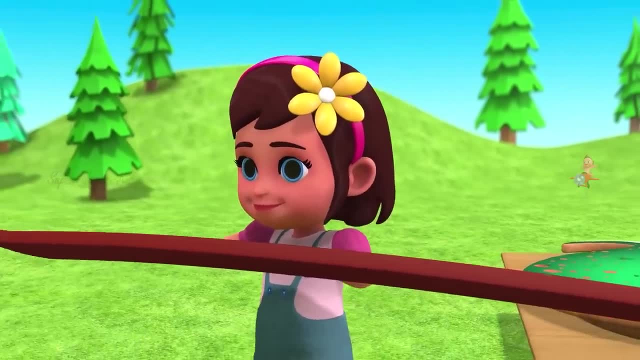 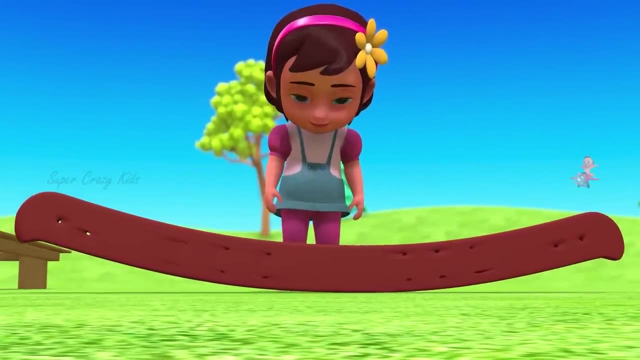 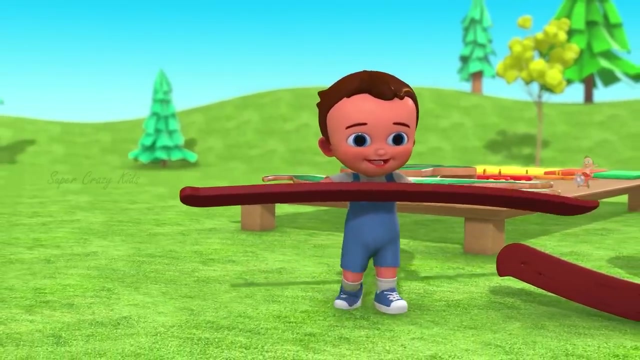 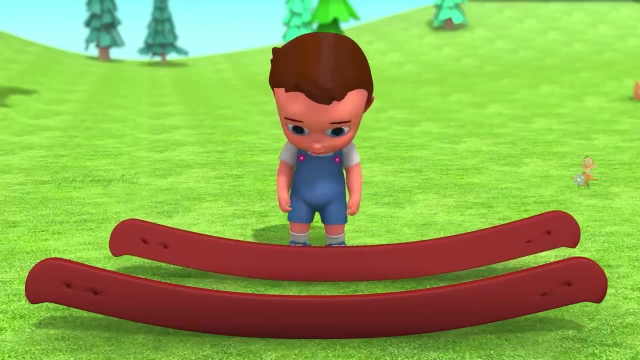 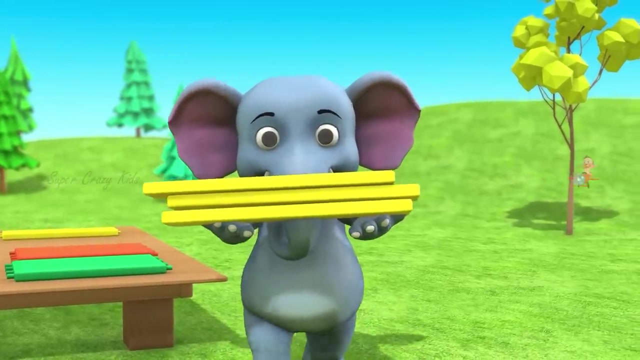 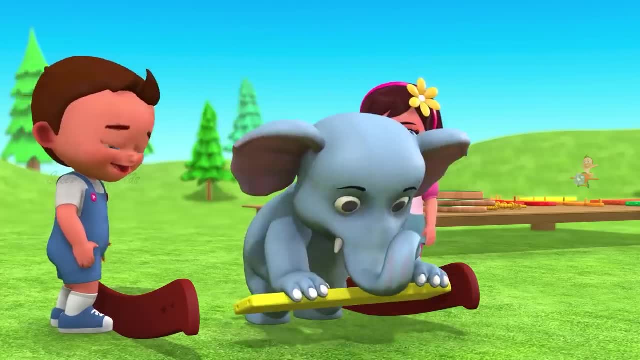 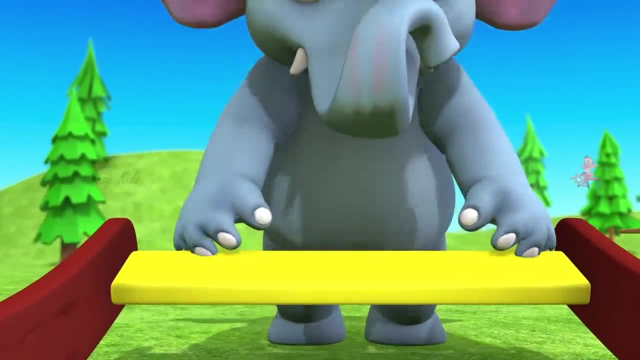 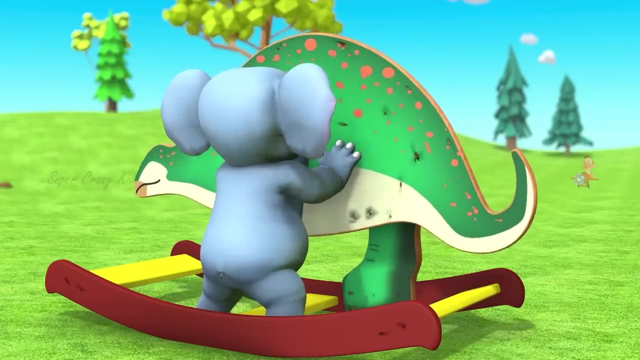 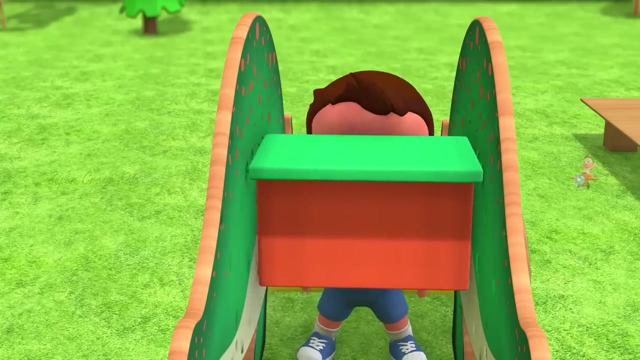 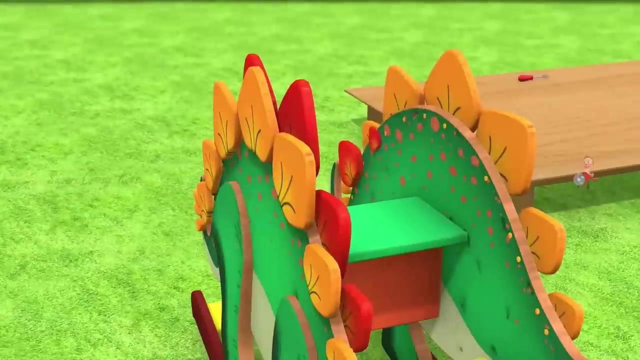 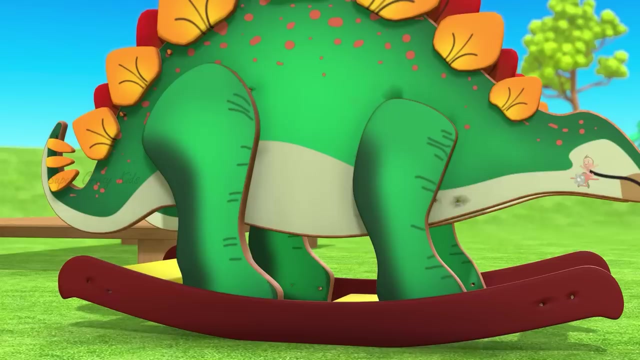 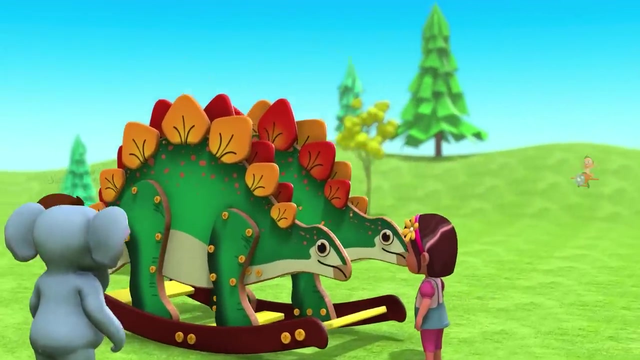 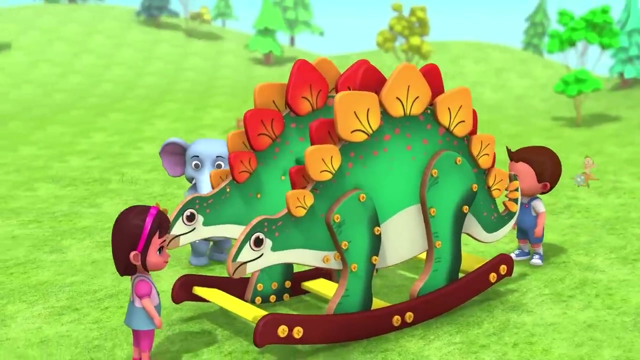 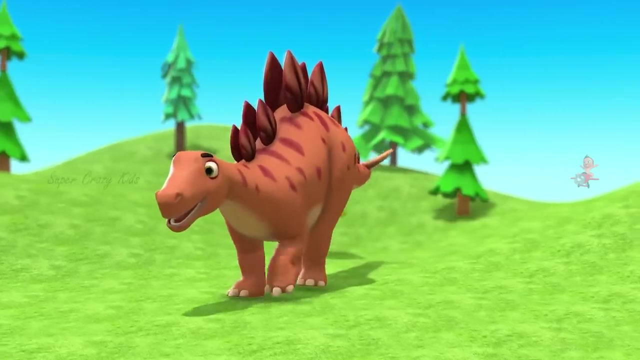 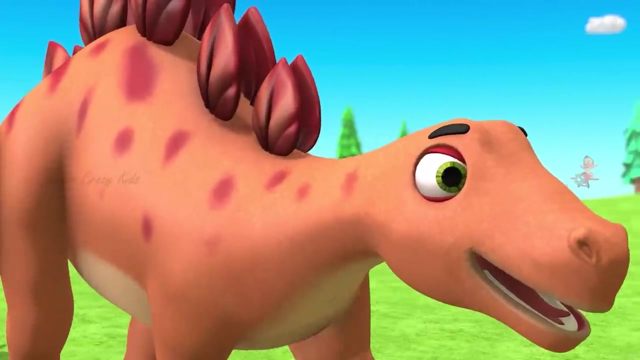 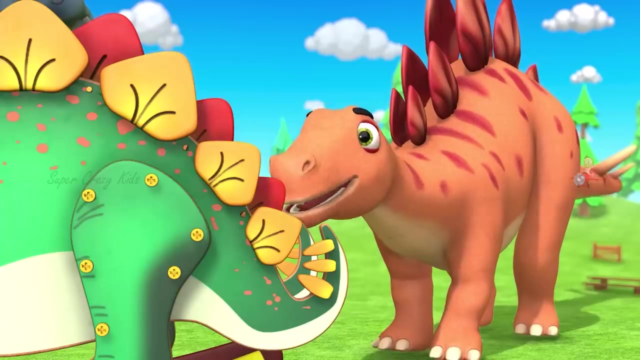 What's up? Perfect, That was wonderful. Thank you, That looks fantastic. I'm so proud of you. See Who was that? That's a Stegosaurus. That is awesome. Do you think you could help today? Here we go, Yahoo. 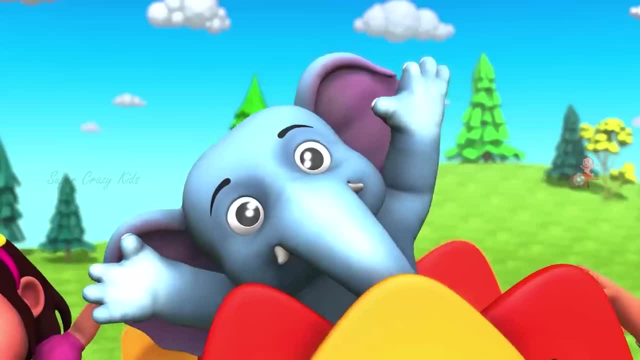 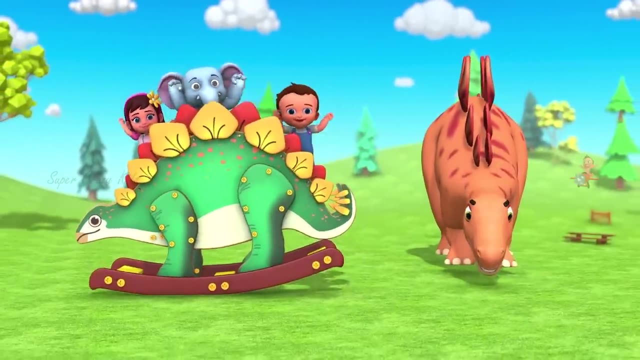 Woohoo, Woohoo, Yeah, Whoa, Ooh, Ooh. So I'm. I will see you next time. Bye.